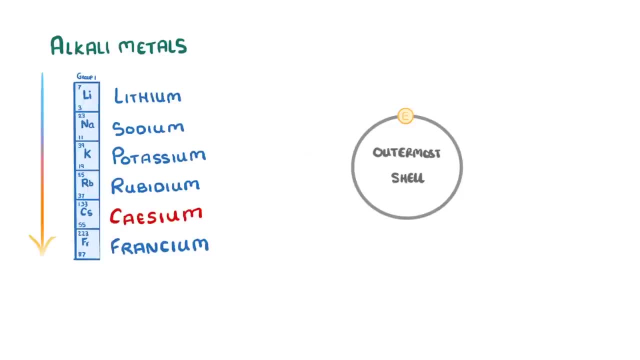 in the outermost shell. So, in order to react and be stable, all they need to do is lose that one single electron, Which is pretty easy because there's only one electron to lose. And because they lose a one negative charge, they become a one positive ion. 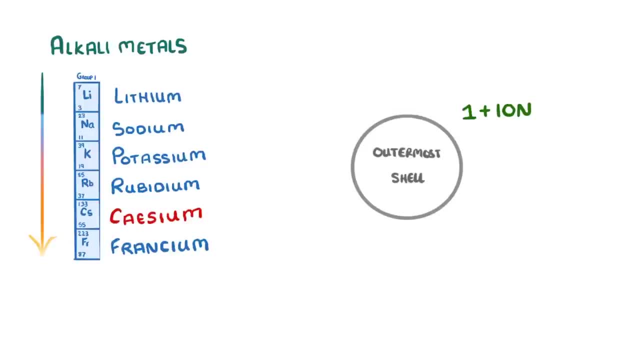 What about the trend that we mentioned, though? That they become more reactive? Well, as you go down the group, the atom's radius gets bigger, and so the outermost shell gets further and further away from that positive nucleus. Now, as this positive nucleus is the only thing holding the outermost electron in place, the 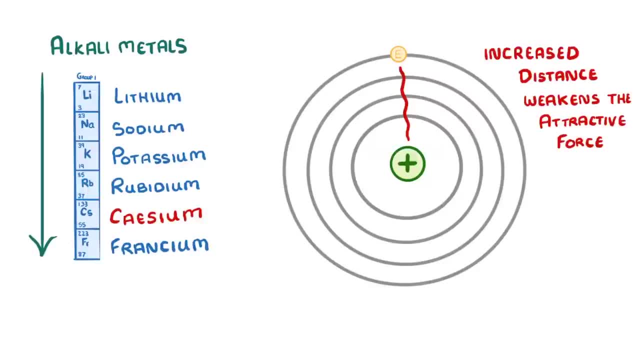 increased distance weakens the attractive force between our positive nucleus and that outer negative electron, meaning that the electron can be lost more easily, increasing the atom's reactivity. Remember this is just a theory. Remember the term reactivity isn't anything special, it's just related to how easily 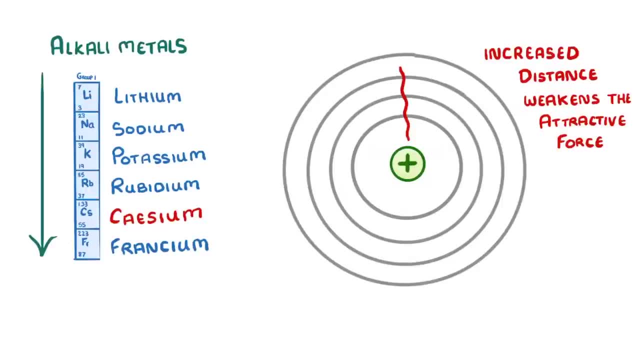 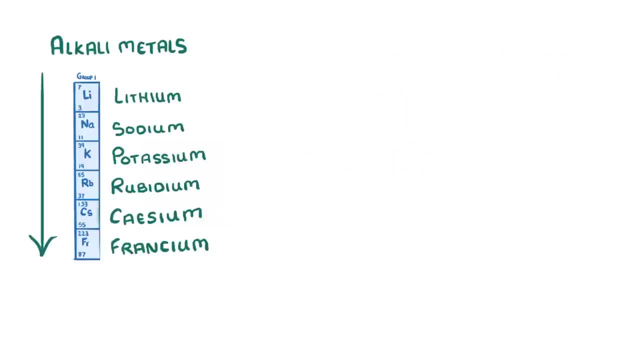 atoms can lose or gain electrons and so react with other atoms. Because alkali metals can lose their outer electrons so easily, they almost always form ionic compounds with non-metals. We'll take a closer look at ionic compounds in another video, but it's basically where. 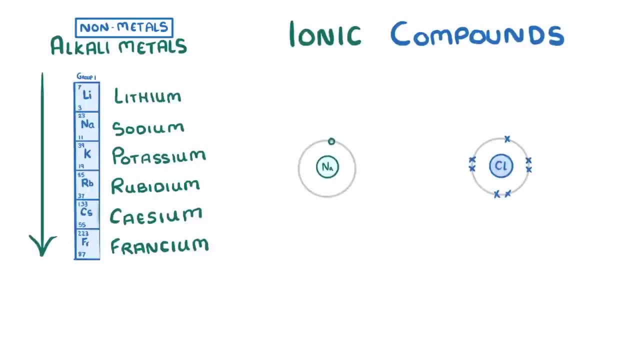 a metal atom like sodium donates an electron to a non-metal like chlorine, so that both of them have full outer shells. And because these two atoms are now oppositely charged ions, they'll be attracted to each other by electrostatic forces, which we call an ionic bond, and so together they make an. 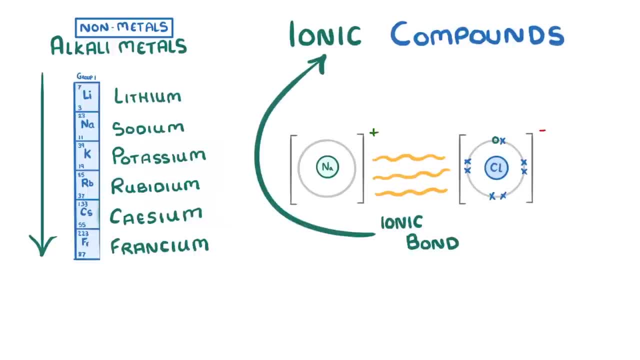 ionic compound. This particular example of sodium chloride actually happens to be common table salt, but regardless of the alkali metal used, the ionic compounds are generally white solids and they tend to dissolve in water to form colourless solids. This is because sodium and chloride are both ionic compounds and they tend to dissolve. 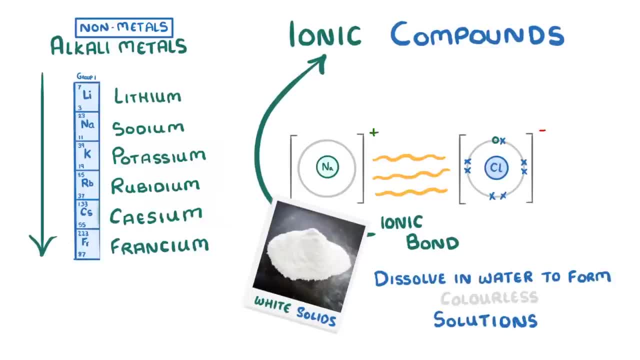 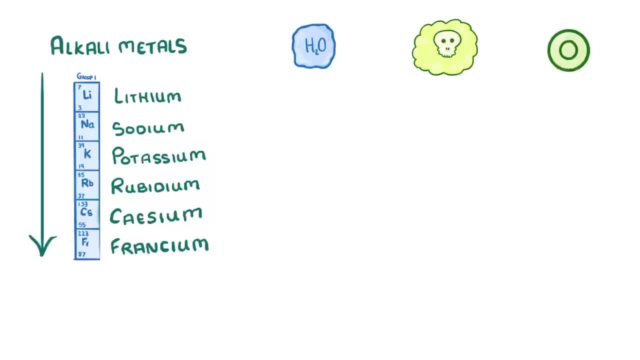 in water to form colourless solids. So now that we've covered alkali metals in general, we need to consider how they react with water, chlorine and oxygen. When an alkali metal is put in water, it reacts vigorously to produce a metal hydroxide and.